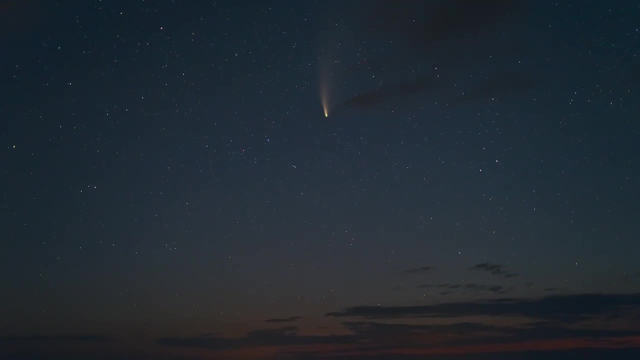 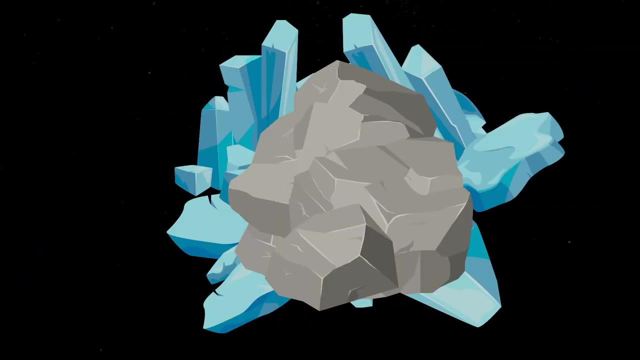 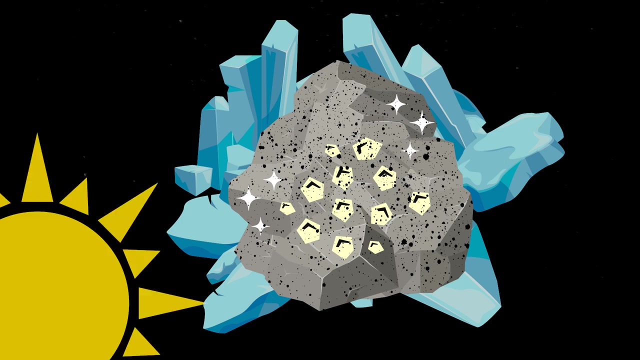 That's kind of what a comet in the sky looks like. Comets have an icy middle which is made up of water and gases that are frozen. They are mixed with bits of rock and metal and are covered by a layer of black dust. When a comet gets close to the sun, the heat from the sun causes the ice to melt and change into a gas. 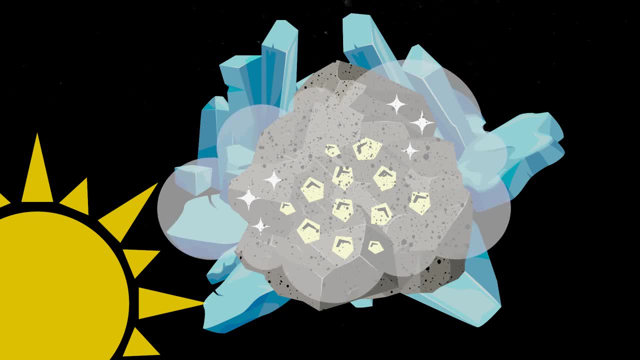 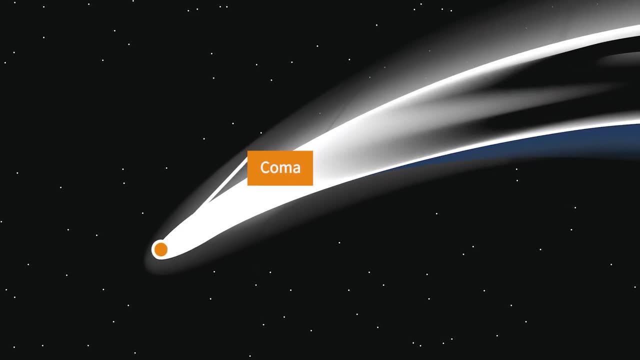 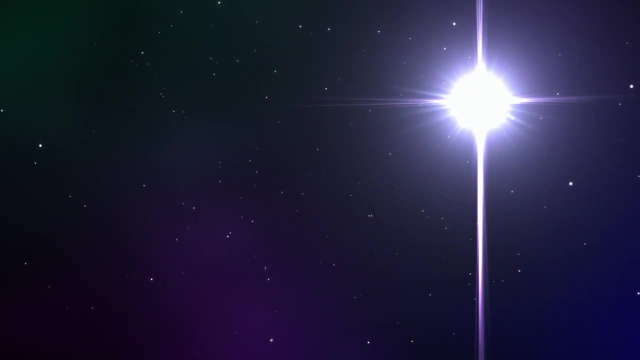 Dust particles spread out around the center of the comet or the nucleus. These dust particles create a cloud at the head of the comet, called a comma. Comets are pretty cool because they don't just shine as one big ball, like a star does. 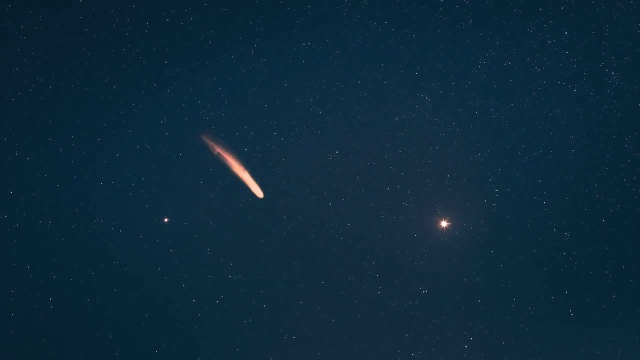 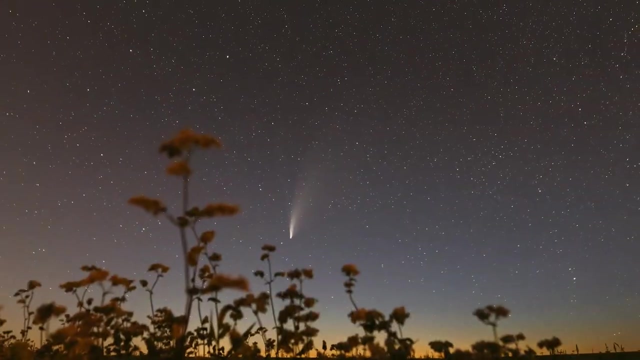 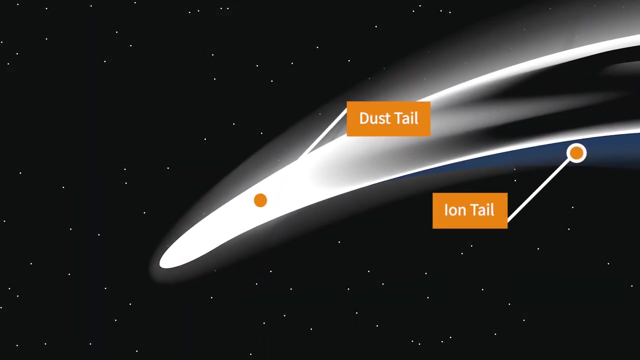 Comets have tails, and these tails shine too. In fact, the tail of a comet is actually the most visible part of a comet. The sun shining on the comet is what causes it to glow. The tails are called dust tails and ion tails. 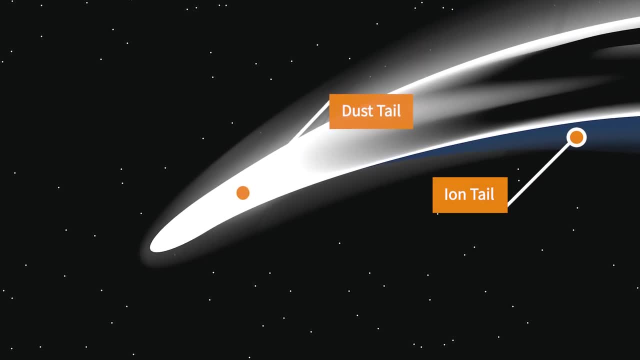 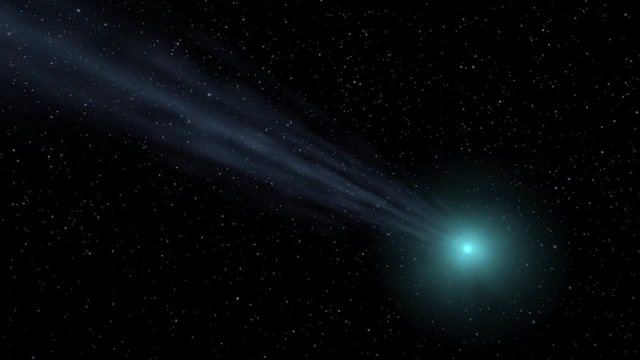 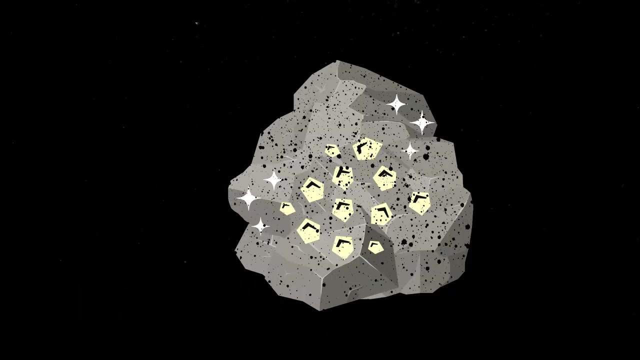 Some tails can be millions of miles long. The tails are made up of gases and tiny dust particles that are blown away from the nucleus by solar wind. How are comets formed? Particles of dust coated with water, ice and other molecules are the beginning of a comet. 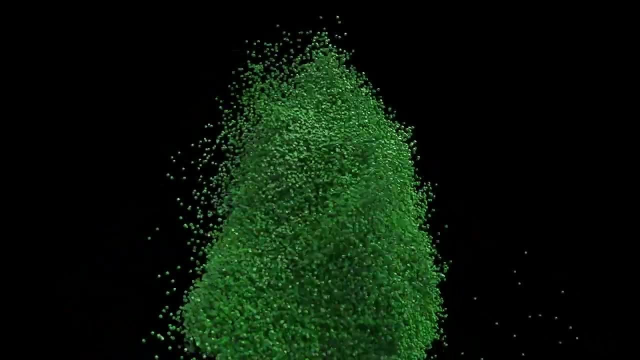 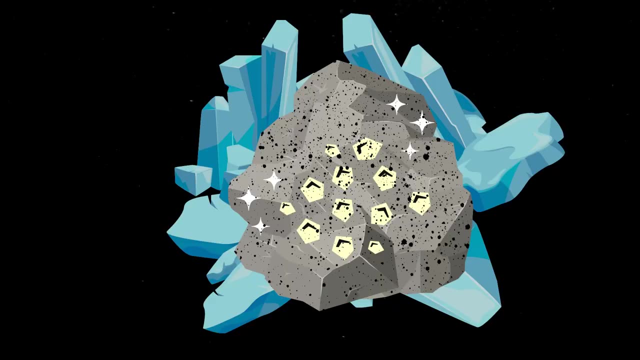 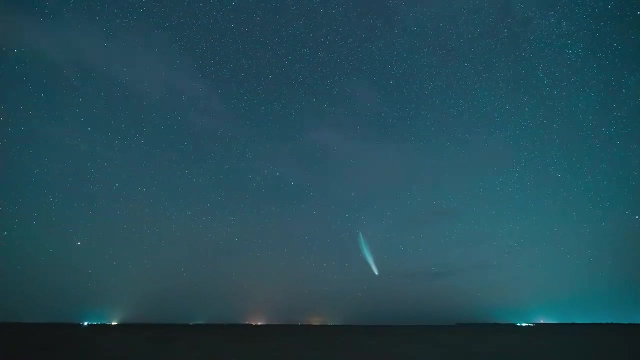 When the dust particles combine, it's kind of like Legos that keep getting stacked on top of each other. Eventually, the combined dust particles form icy rocks. Gravity then pulls those icy rocks together and you get a comet. Where do comets come from? 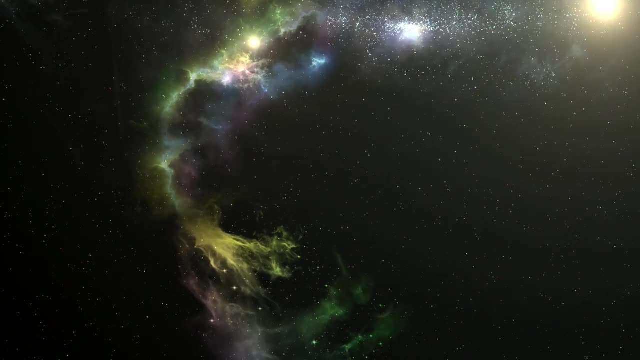 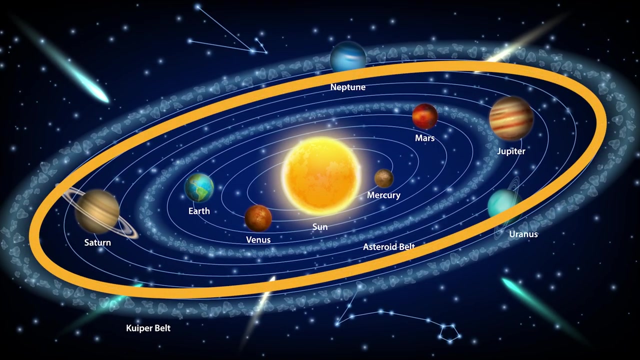 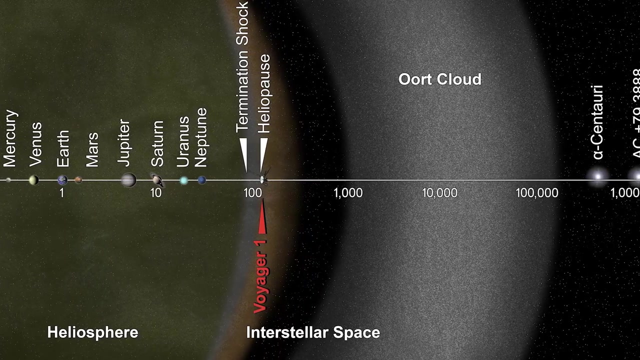 Comets come from two places in the solar system. The first place is called the Kuiper belt. The Kuiper belt is just beyond the orbit of Neptune. The second place is called the Oort cloud. This region is farther out than the Kuiper belt, so comets from this region take longer to orbit the sun. 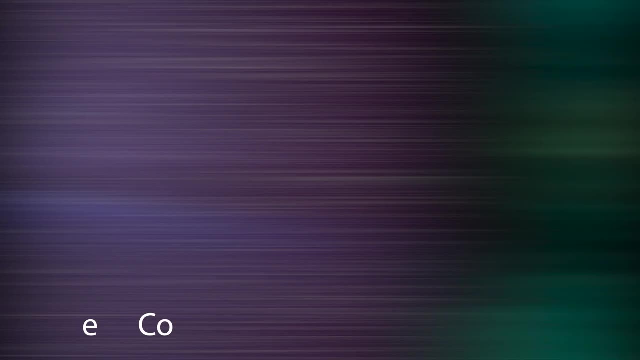 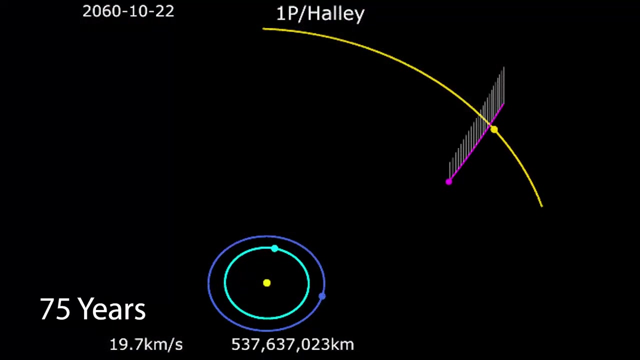 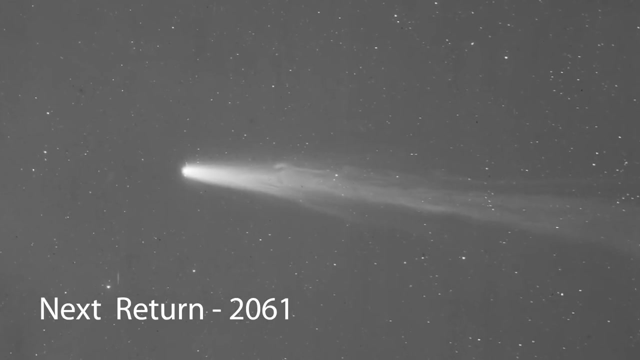 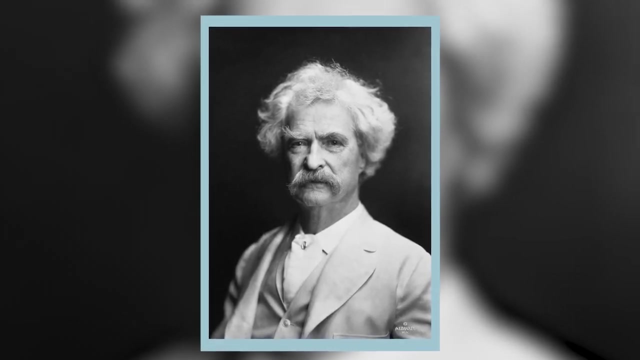 Are there any famous comets? You betcha? Halley's comet is one of the most famous comets. This comet is visible about once every 75 years. Scientists predict that it will next be visible in the year 2061.. Famous writer Mark Twain once said that he was born on the day that Halley's comet passed by.